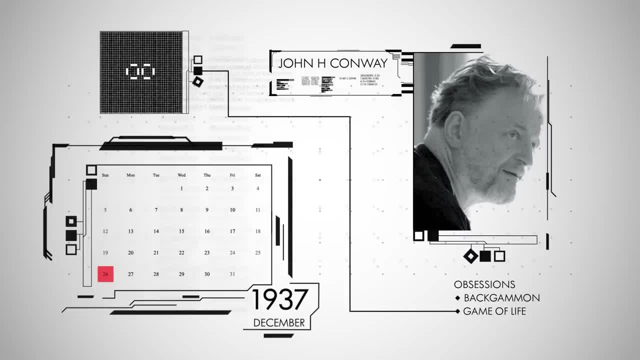 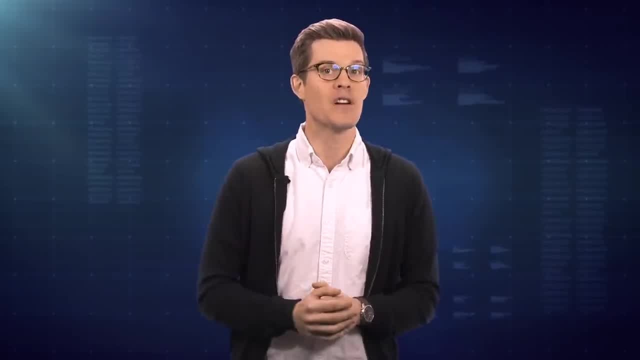 famous Game of Life, a machine that follows simple rules but can evolve incredible complexity. He can also tell you the day of the week for any date past or future in a couple seconds. Conway's smart, but he hasn't memorized thousands of years of calendars. 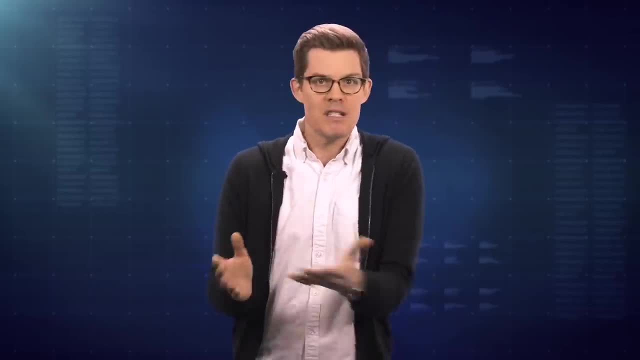 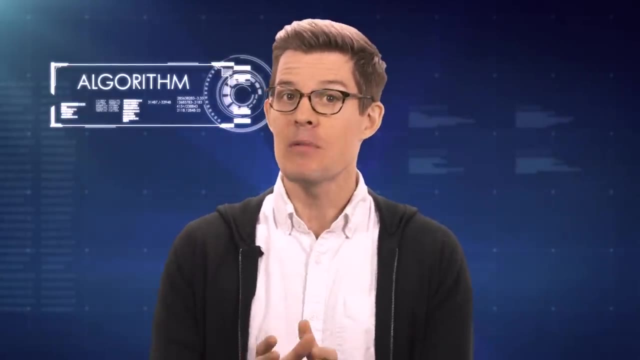 He figured out how to answer this complex question with a simple set of rules. He invented an algorithm After watching this video. with a little bit of practice, you'll be able to do it too. All with just one hand. Alright, gimme a date. 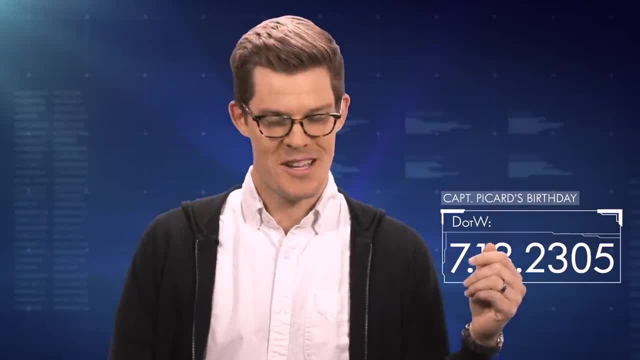 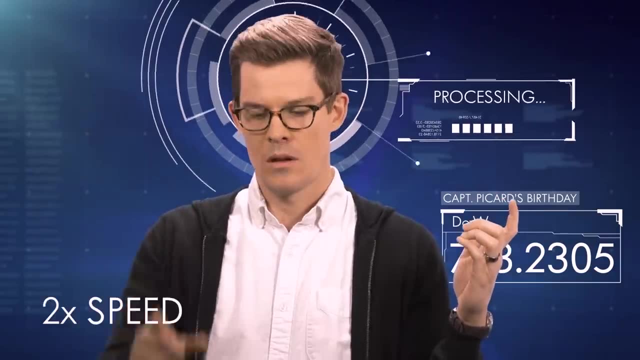 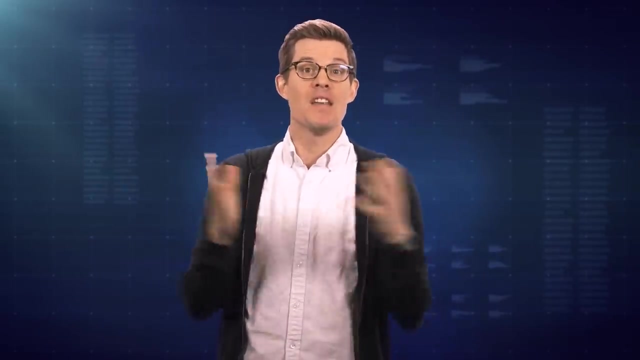 July 13th 2305.. Whew, July 13th 2305.. Okay, um… That is a Thursday, Correct? Yes, Alright, here's how it works. First, let's give the day of the week a number. 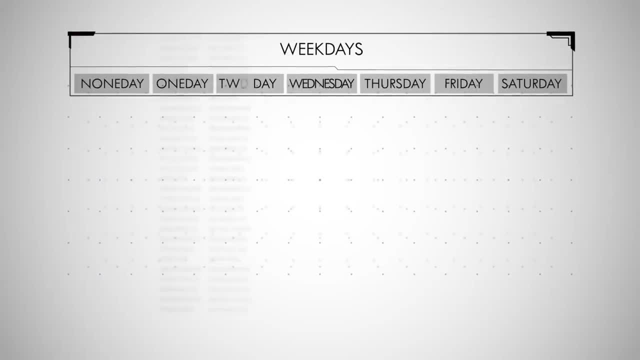 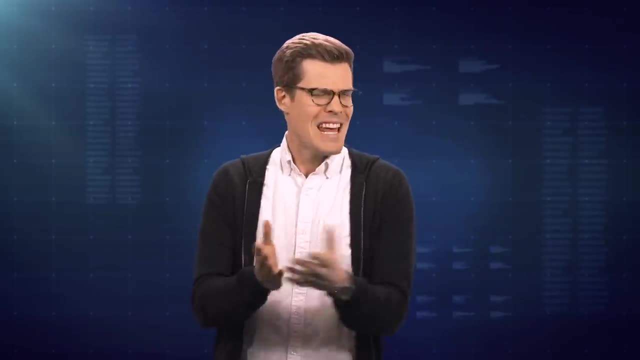 Here's an easy way to remember them: None day, one day, Tuesday, three's day, four's day, five's day, six's day. We'll use this in a sec. Next, Conway realized that, in any given year, specific dates always share the same day of. the week April 4th, always the same weekday as October 10th. We can make another easy list. For even-numbered months it's the same date as the month, Unless it's February, when it's the last day of the month. 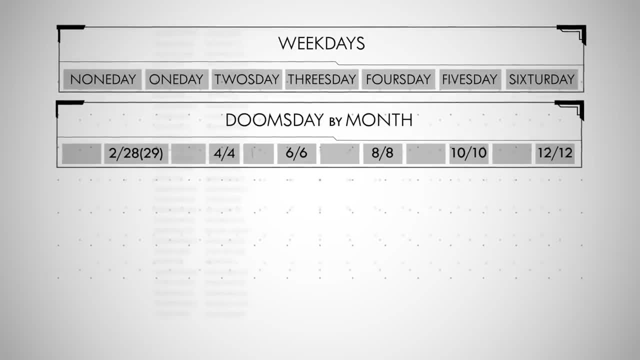 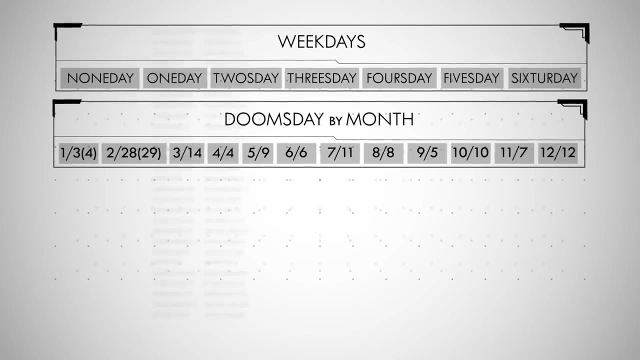 The odd months are a little less obvious, but just remember, I'm working 9 to 5 at the 7-11, and you're almost there. All that's left is Pi Day and January, which is the third, unless it's the fourth in a leap year. 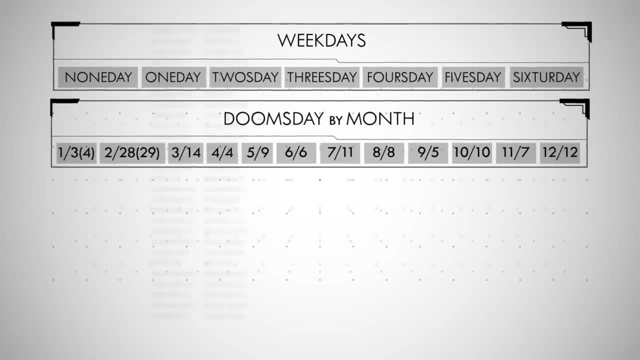 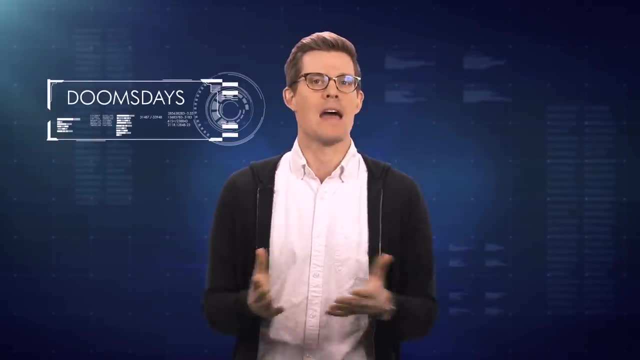 And now we've got our list, a set of dates that are the same day, one every month. These are what Conway called Doomsday- Scary name but relatively easy to memorize. And since weekdays repeat by sevens, we have a reference for any day of the year. 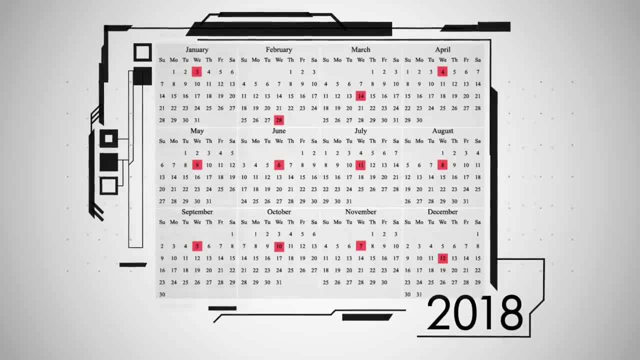 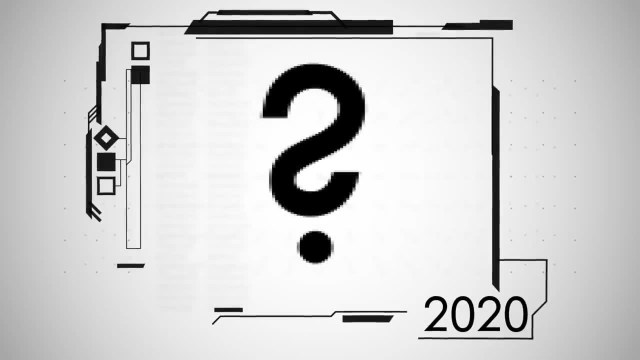 2018's Doomsdays are all Wednesdays, But most years the weekday for a date moves forward one day. So in 2019, Doomsdays will be Thursdays, But 2020 is a leap year and weekdays jump by two. 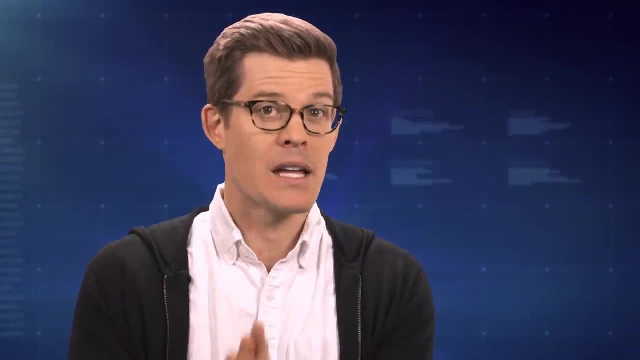 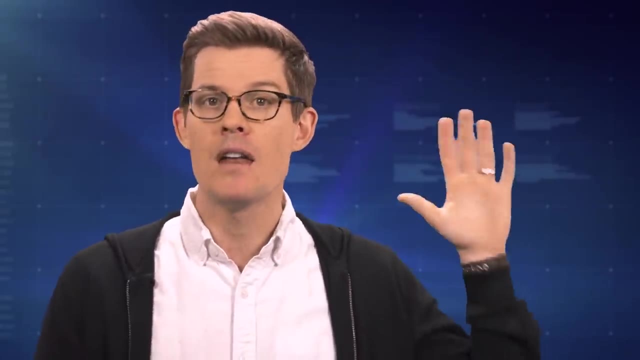 This is getting confusing. We're going to need to find a different way to calculate our Doomsday. First, let's start with the century. 2000's Doomsday was a Tuesday. Let's hold that number 2, here. 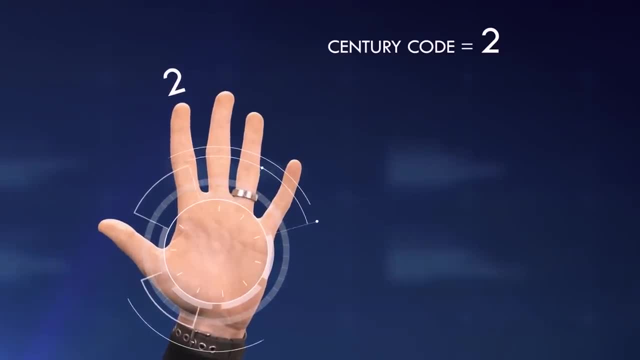 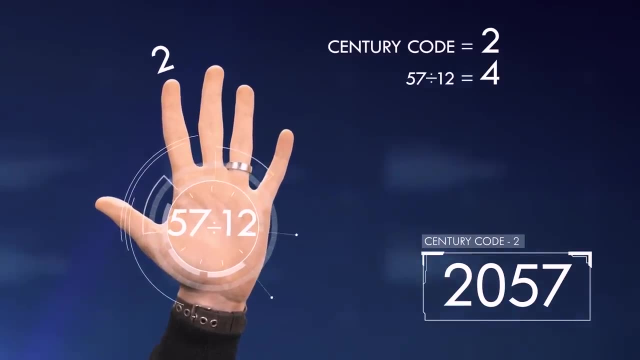 To find the Doomsday for any other year in a century was Conway's stroke of genius: 2057.. First figure out how many times 12 goes into the year 4.. And hold that number here. Put the remainder, 9, here. 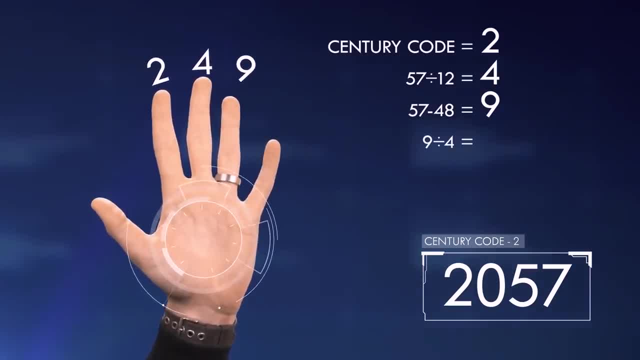 And finally figure out how many times 4 goes into the remainder 2. Put it on your pinky, Add these four numbers. If the number's more than 6, divide 7 into it as many times as you can, and what's left. 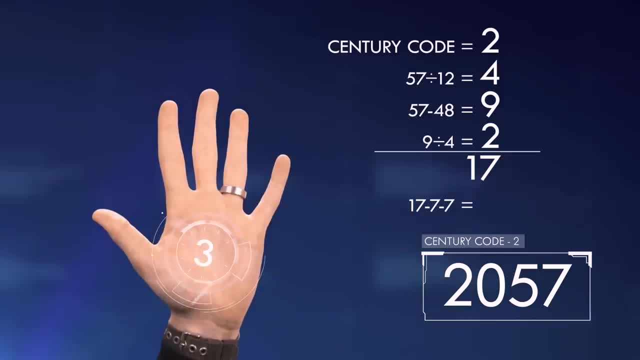 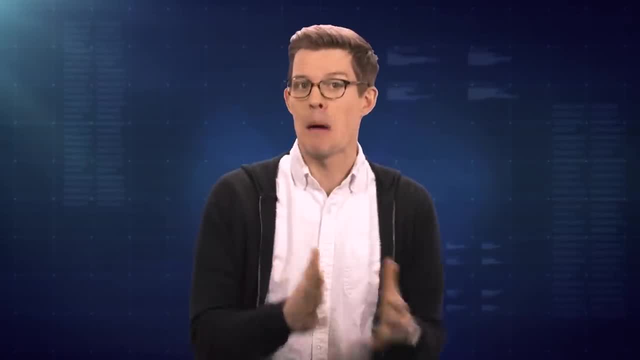 over 17 is 7,, 7, and 3.. Wednesday's the Doomsday for that year, For a different century. we just need to change the index number or century day: 1900?. Wednesday 1800?. 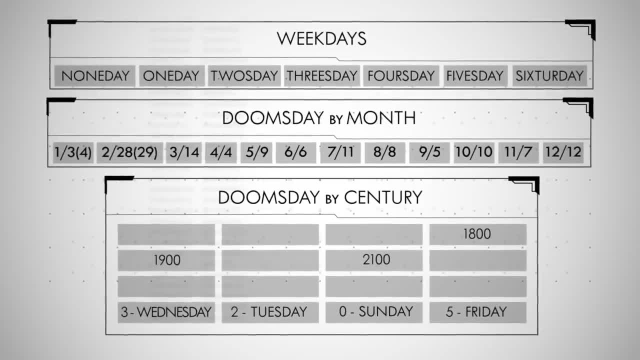 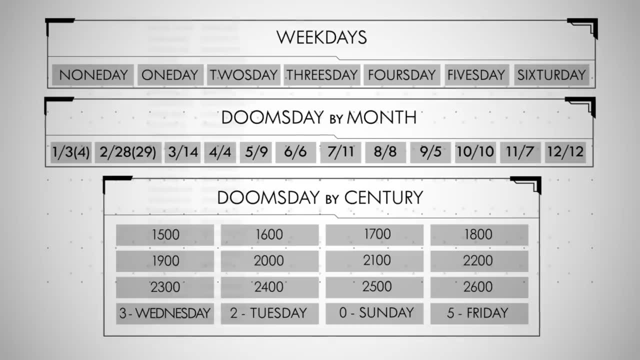 Friday And the year 2100's Doomsday will be Sunday. Since our calendar, the Gregorian calendar, repeats every 400 years, we can figure out any other century just by remembering these. Now we have all we need to figure out the Doomsday for every century. 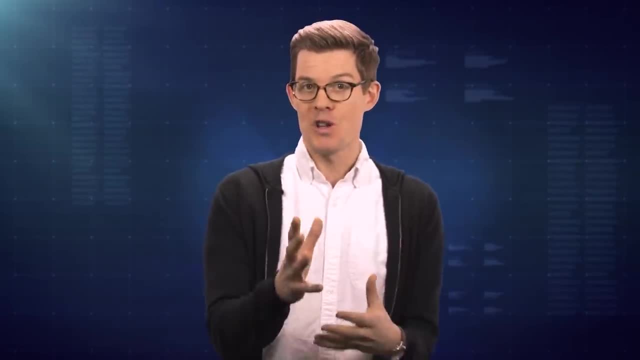 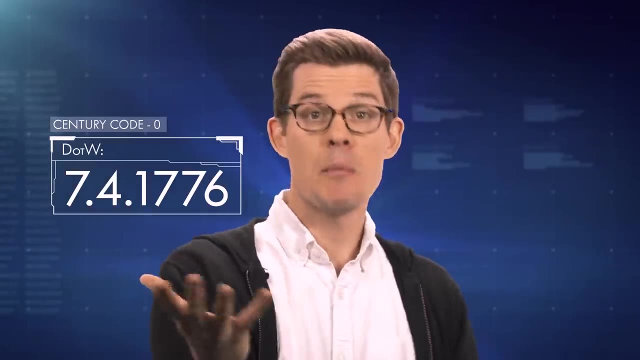 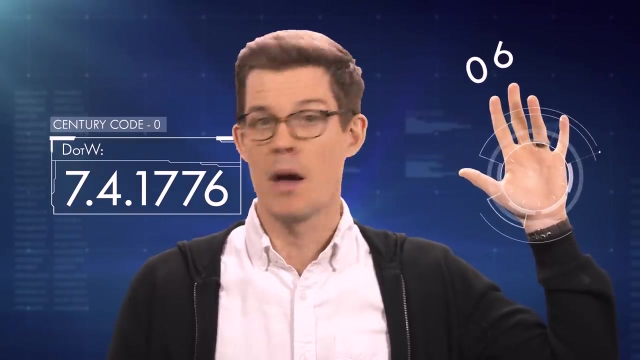 And once we know that we can figure out any other day that year, Let's try. What day was the Declaration of Independence signed Just like 2100, the century code is 0.. 76 is 6, twelves remainder 4, and there's one 4 in the remainder. 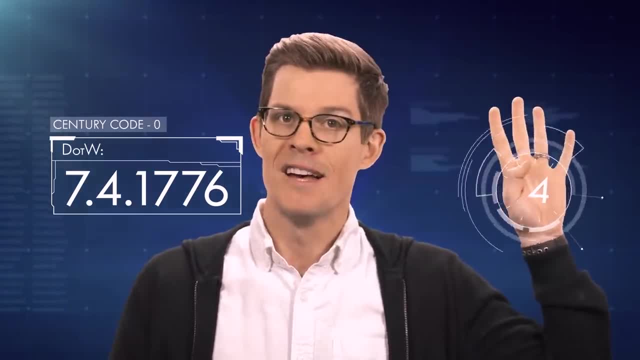 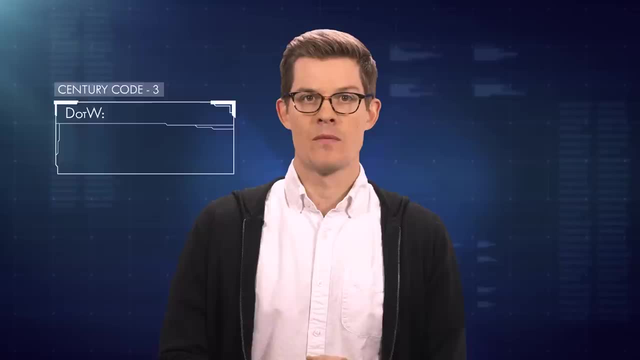 0, 6, 4, 1 is 7 and 4.. The Doomsday for 1776 was a Thursday And since 7-11 is a Doomsday, so is 7-4.. The first moon landing. 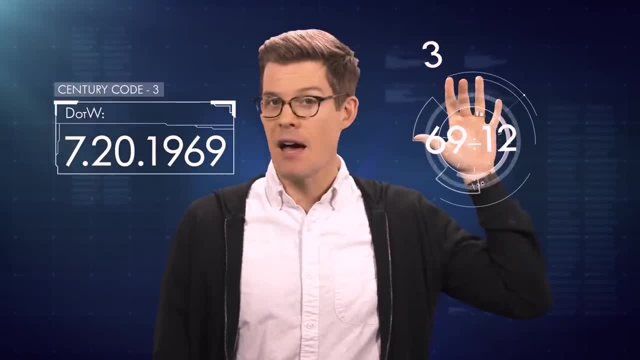 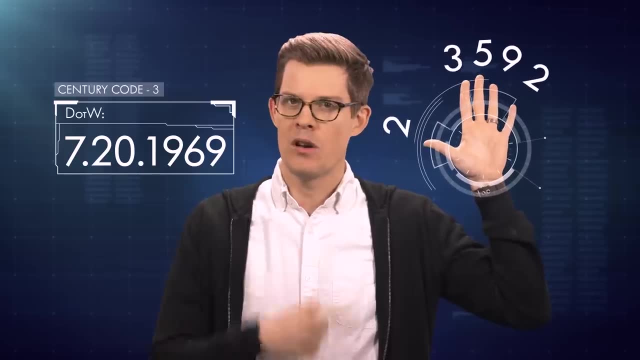 The century code is 3.. 69 is 5, twelves, remainder 9, which is 2. fours. July 20th is 2 days after a Doomsday, so put it on your thumb: 2,, 3,, 5,, 9, and 2 is 7, 7, 7, and 0. 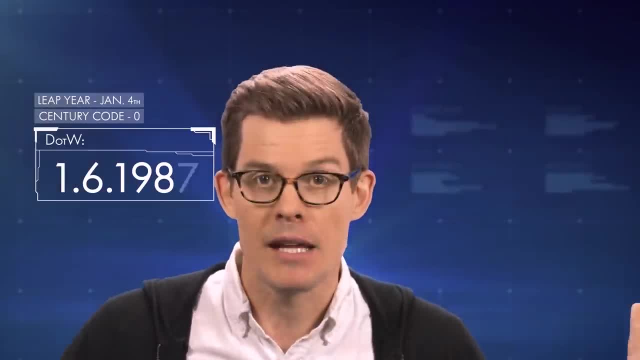 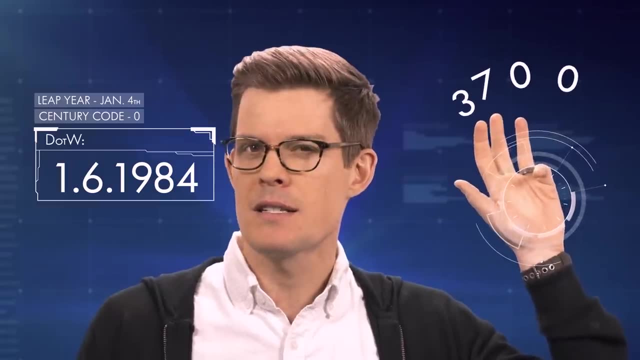 It was a none day: Kate McKinnon's birthday, January 6th 1984.. So that's 3, 7, 7, and 0.. 7, no remainder, no remainder. And since it's a leap year, 2 days after the Doomsday. 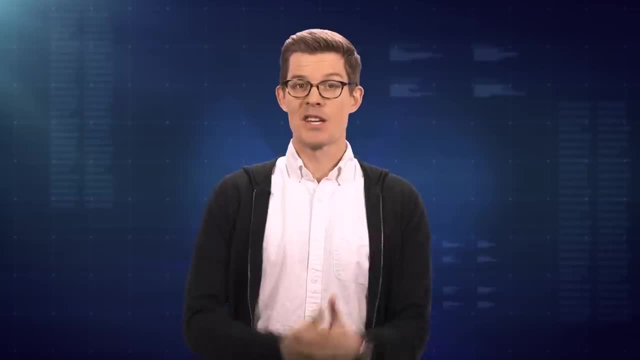 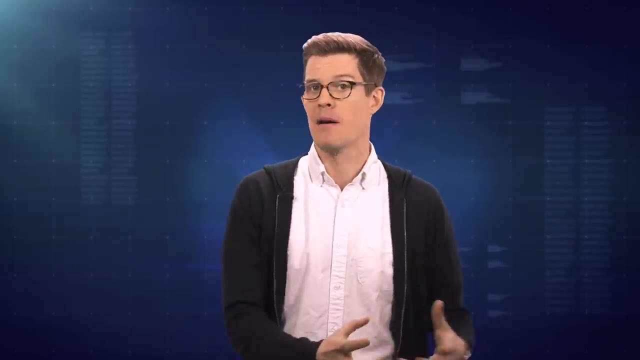 And if you ever meet her, you can tell her she was born on a Friday. Congrats, you just performed an algorithm. Algorithms are a set of instructions for solving a problem step by step. We know them best from computers, but we run algorithms too, all the time. 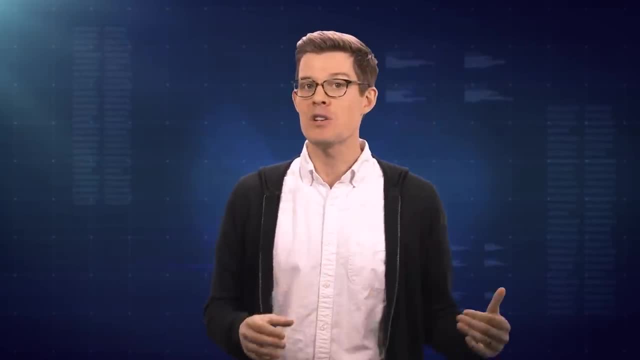 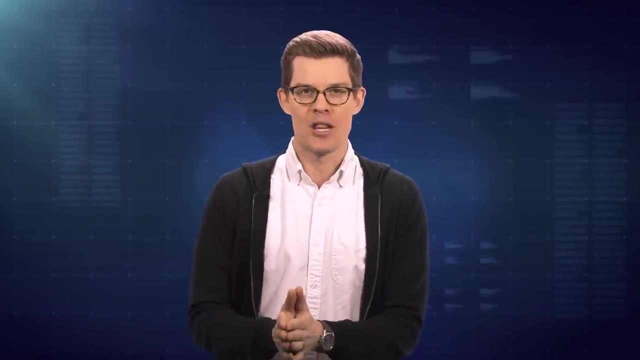 In fact, the word algorithm comes from a Persian mathematician who wrote a book for doing math by hand, The same book that gave us algebra. We're interested in algorithms getting more than just the right answer. We also want algorithms to do things efficiently. 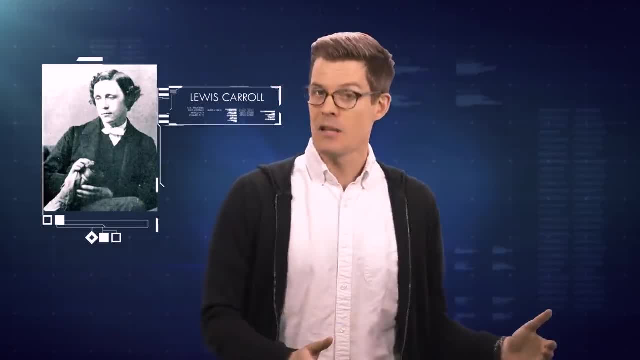 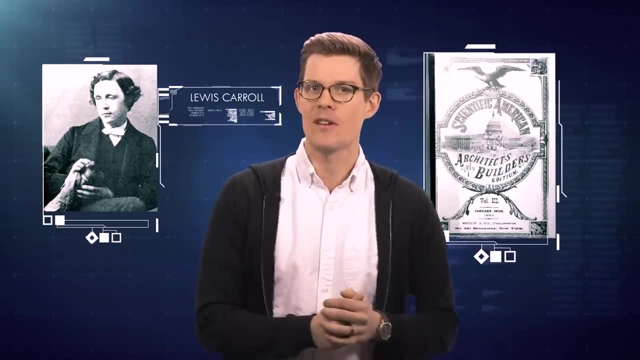 Lewis Carroll, the author of Alice in Wonderland and a mathematician, developed his own algorithm for solving the day of the week. It was printed in Scientific American on June 18th 1887.. A Saturday, But Conway's is quicker. 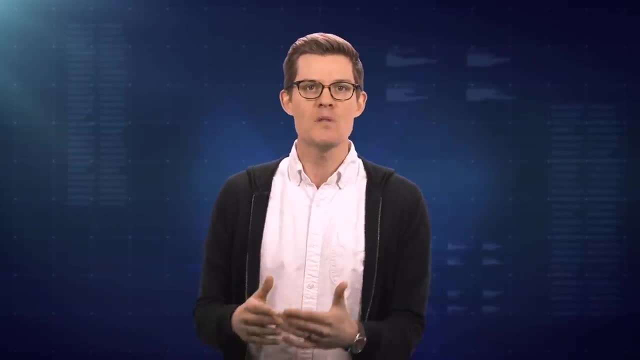 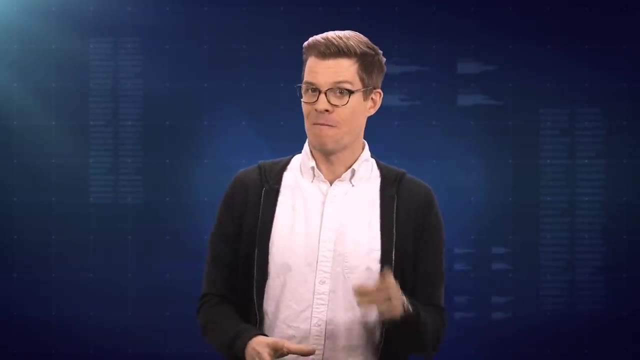 These days, this kind of information is only a few clicks away, But it shows us how the right algorithms can extract answers from even complex data And how, with a little bit of practice, you can be as smart as a computer, At least for one day. 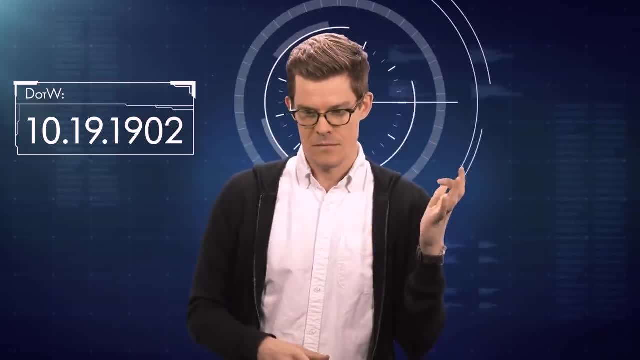 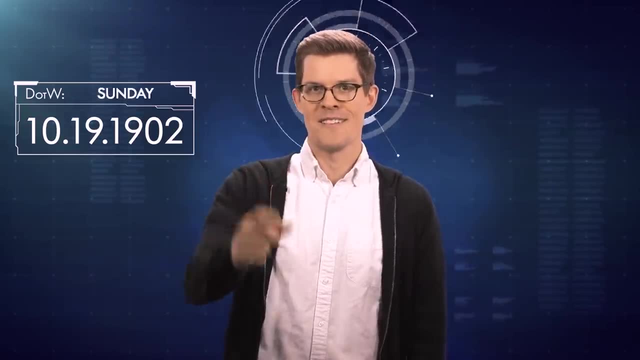 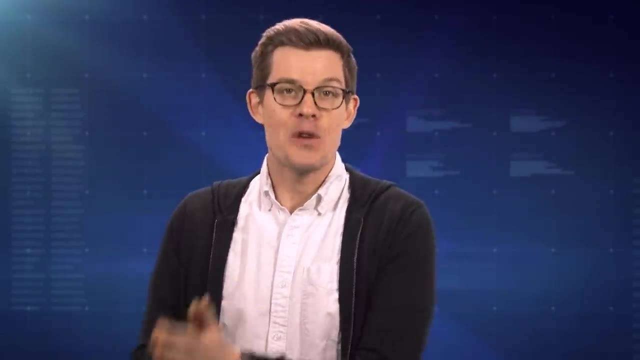 October 19th 1902.. It's a Sunday, Correct. Stay curious If you're sitting there thinking there's no way I could do that. Trust me, if you can do arithmetic, then you can. I've been practicing this method for a few days and now I can calculate any date at any time. 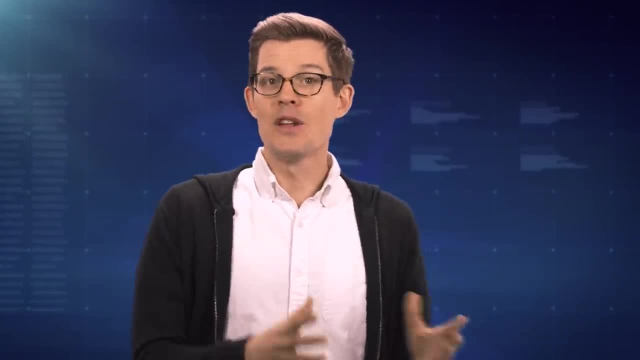 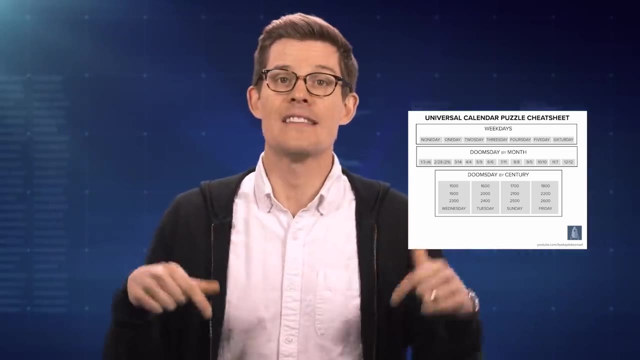 Any date in a handful of seconds, and I'm usually right. If you'd like to practice, we made this cheat sheet for you, And there is a non-US version too, because I know we write dates funny. There's a link to that down in the description. 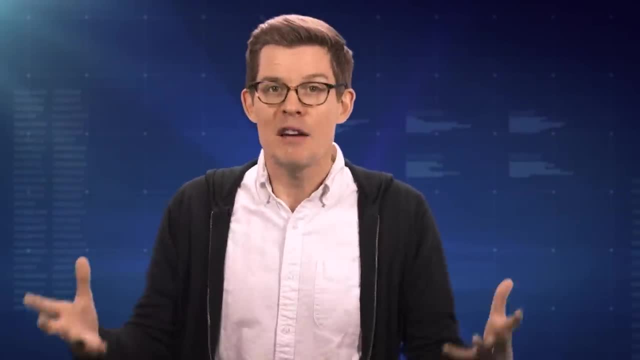 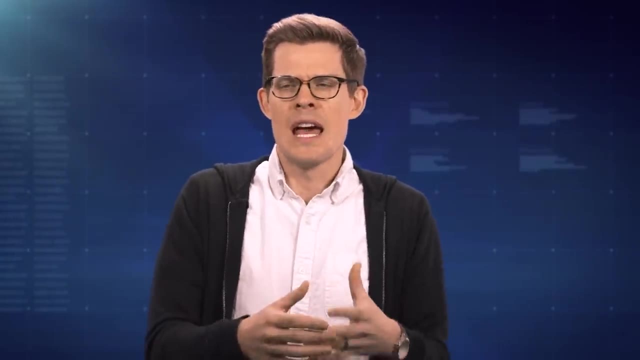 I hope I've sparked your curiosity and showcased the beauty and fun of mathematics. When I was preparing for this, I couldn't simply memorize this formula. I had to critically reason it through to understand how and why all the various parts fit in, so I could explain it clearly. 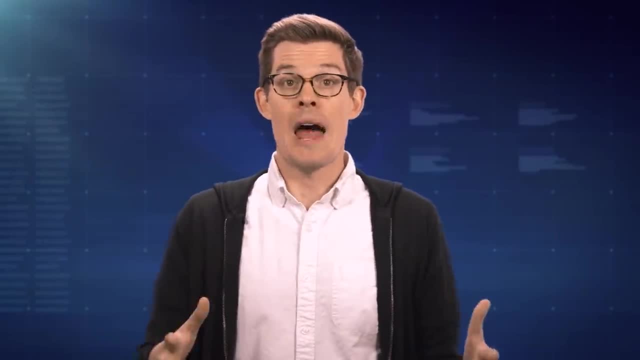 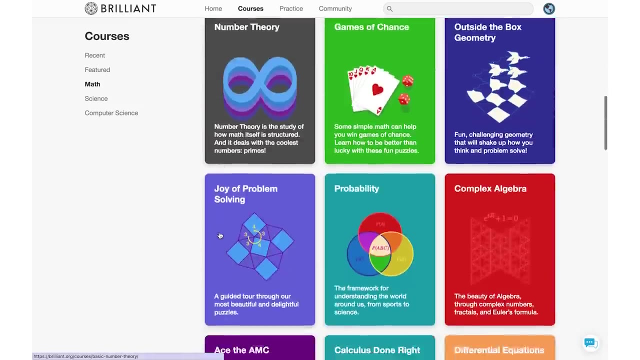 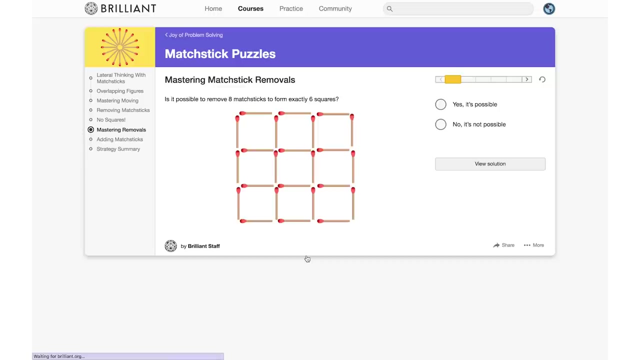 If you'd like to sharpen your brain and develop these tools, then Brilliant could be the place to go for that. You don't just watch stuff, You actively do stuff. I enjoyed their Joy of Problem Solving course. It presents fun puzzles that are cut up into easy-to-digest bits.